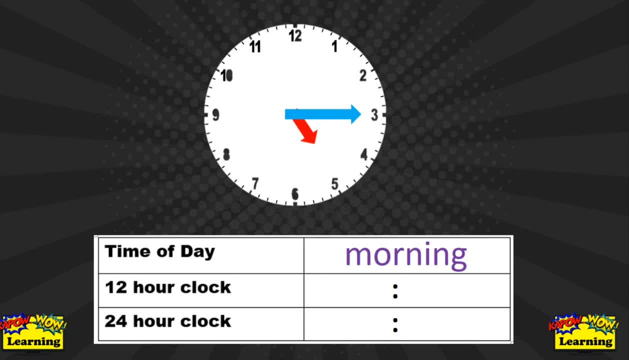 and 10 minutes. 10 minutes past three. Let's have a look at the next time. You can pause this, then try to answer Right. how many hours is on that? We're in the morning here, so we need to be careful. 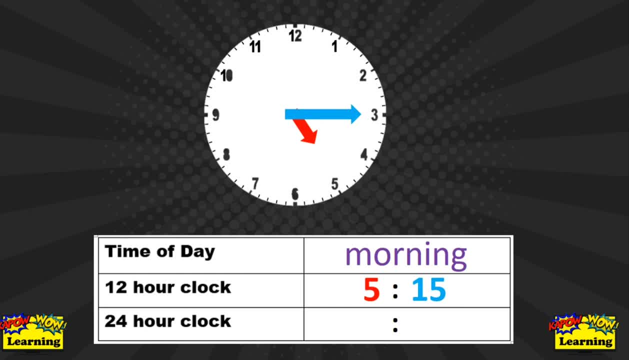 So it's five hours and 50 minutes, okay. And because it's the morning, we always have to have two digits in the hours column. So we do zero. five hours and 50 minutes. The minutes remains the same. What time is this? You can pause this then try to answer Right the hours here. it's still the. 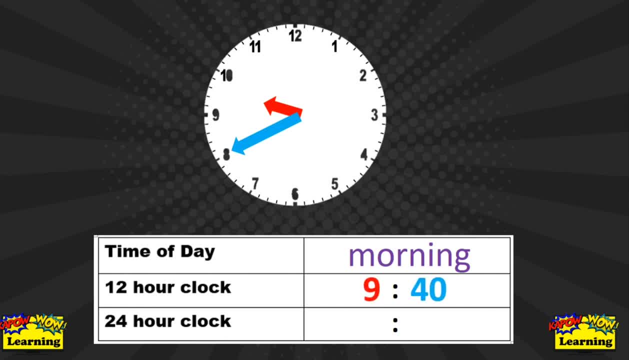 morning. So we've got nine hours and 40 minutes. okay. So we don't just write nine hours, We have to have two digits in the hours column. So we write zero, nine hours and 40 minutes, 9.40 or 20. 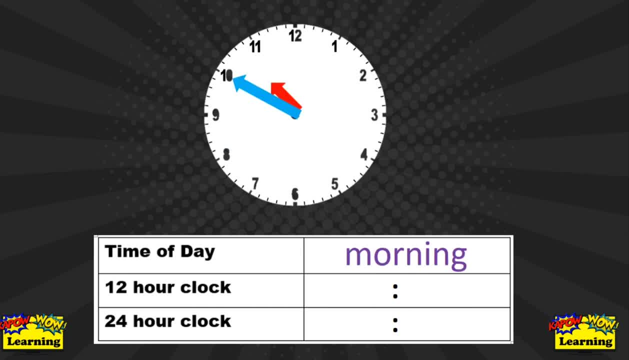 to 10, you could say What time is this. You can pause this, then answer: It's in the morning, Right? so the hours is 10.. Hours and how many minutes? 50 minutes, okay, And for 24 hour clock because it's the morning. 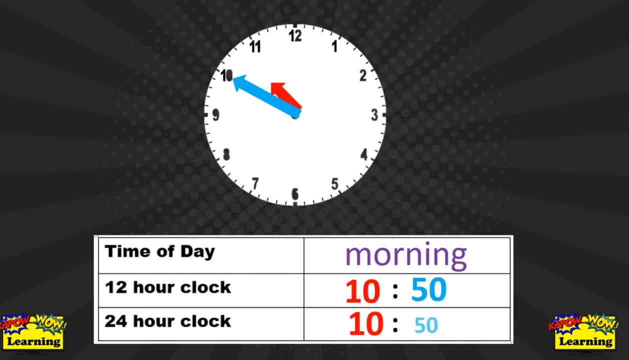 we just write 10, because there's two numbers there Remains the same in the hours and 50 minutes stays the same. Now, this time we're in the afternoon, so you can pause this, okay. So in the afternoon you need to be careful. Pause this, try to answer So the hours you should. 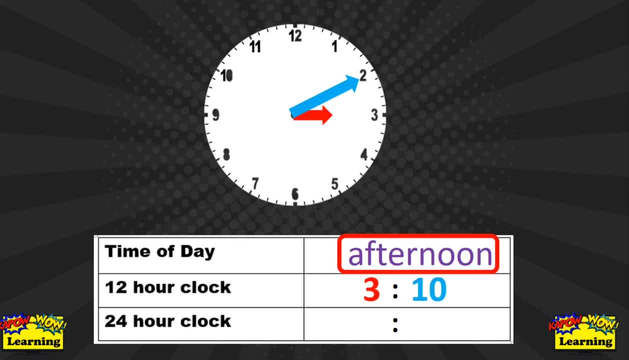 have had three hours. How many minutes? Right now? because it's past 12 o'clock in the day, we need to add 12. 12 hours to the hours. So 12 plus three is 15 hours, and again the minutes remains the same. So 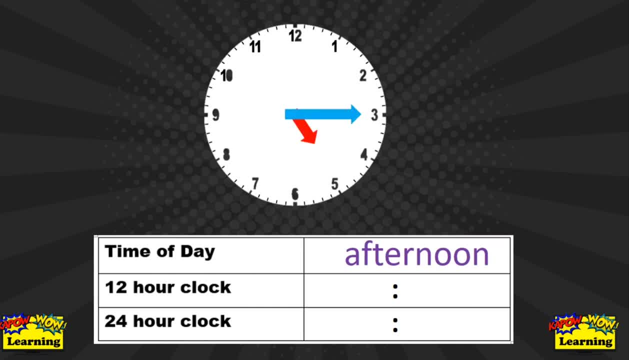 15 hours and 10 minutes. 10 minutes past three. What time is this? You can pause this and then answer it again. Right, so this is the afternoon. How many hours is there? You should have said five hours and how many minutes? 15.. Excellent, And what time would this be on a 24 hour clock? 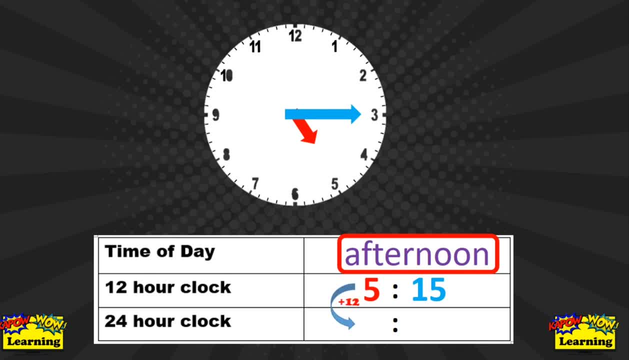 Right. so because it's past 12, we're going to add 12.. So 12 plus five is 17.. So that would be 17 hours and 50 minutes or quarter past five. you could say What time is this? You can pause this, then answer Right, you should have had now. this is in the.